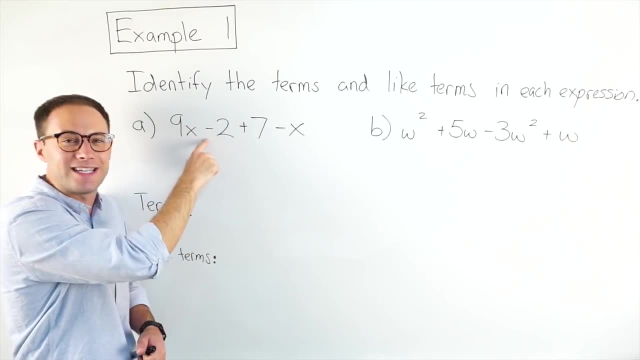 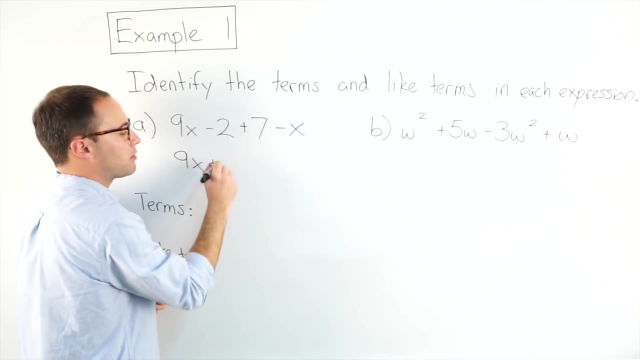 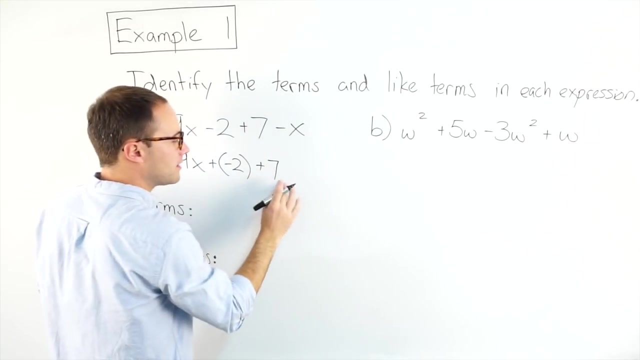 I have subtraction. I'm going to change that to addition, adding the opposite. I'm going to rewrite this as nine x instead of minus two. I'm going to say plus a negative two and then plus seven, that's okay, And then instead of minus x, you probably could guess it- plus negative x. So 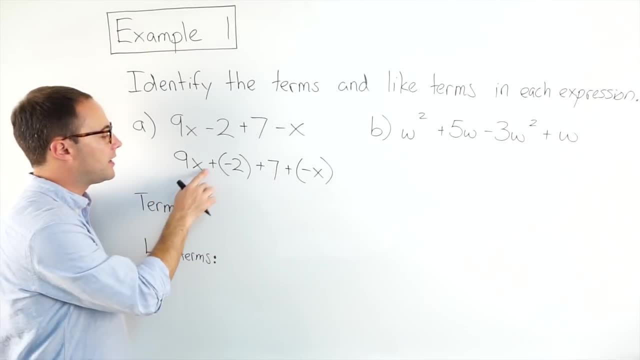 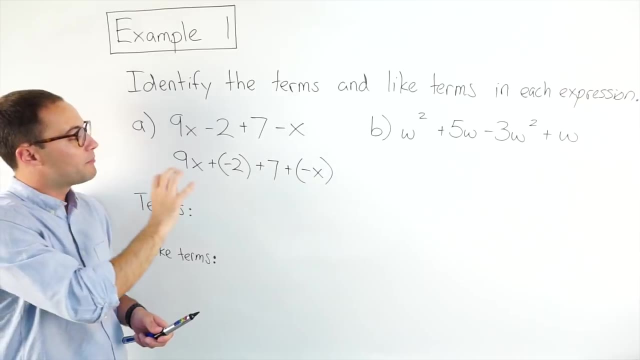 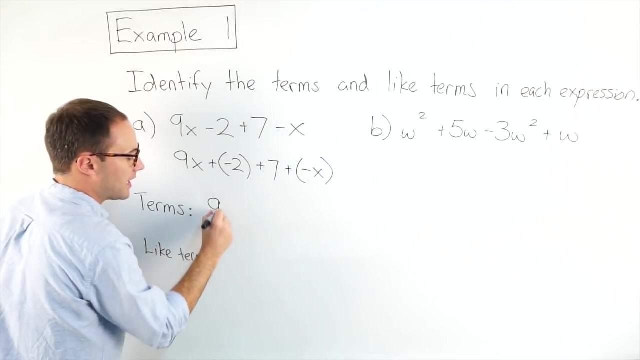 my first step is just to rewrite the expression as an addition expression. Now I'm ready to identify the terms. And again, the terms are the parts of the expression without the operations. So the terms that are: nine x, negative two, seven and negative x. those are my terms. 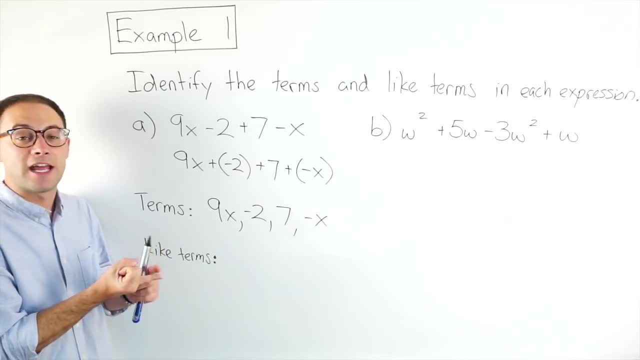 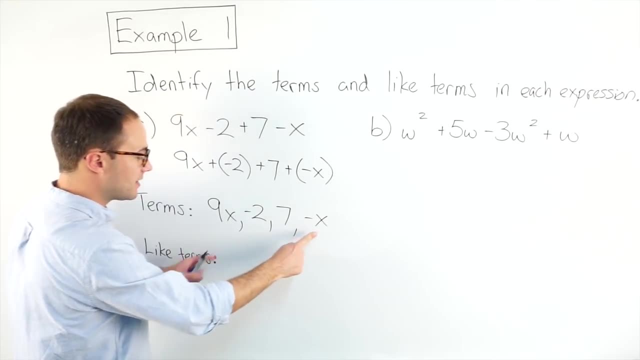 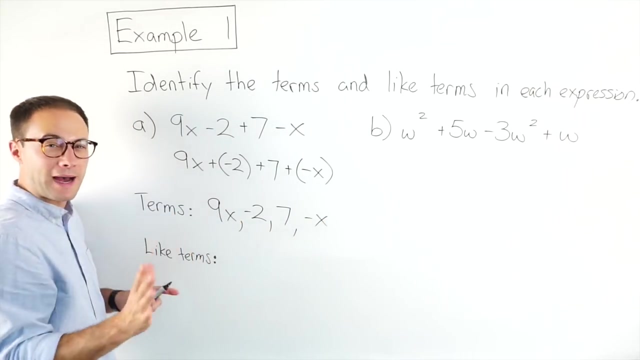 my like terms are where I have the same variables raised to the same exponents or constants. I have a nine x and a negative x. they're both x. it doesn't matter that this is negative, that's okay. The fact is that both of these are raised to the first power, even though 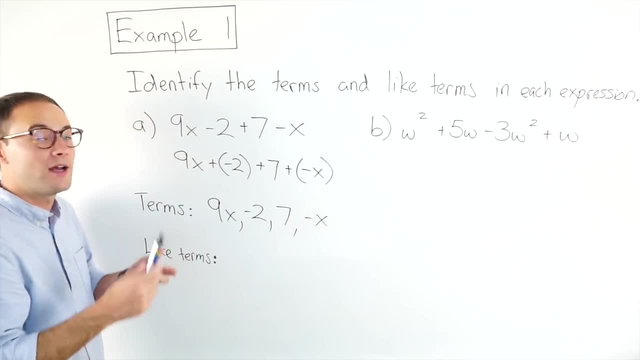 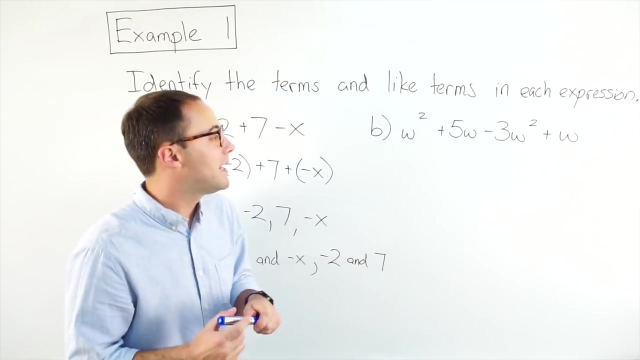 we don't write it. there's just one x, Okay. so those are like terms nine x and negative x. Now I'll put a comma. my other group of like terms are my constants: negative two and seven. negative two and seven. Okay, part B. 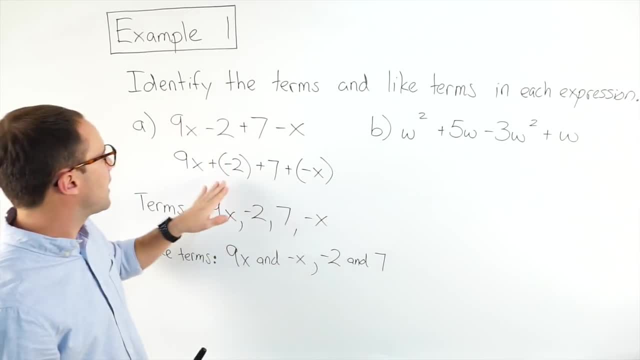 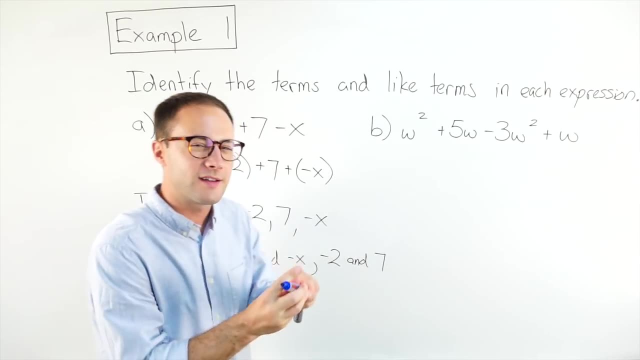 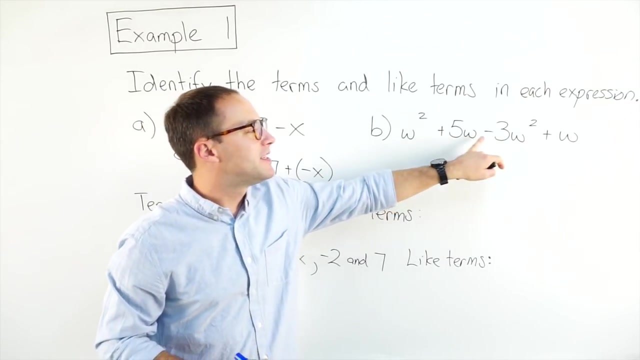 I'm going to do slightly different. I could do the same thing and just change it first to an addition expression again, But I'm going to circle, and this is another strategy that a lot of students like to use. You just circle the parts of the expression And if you see a negative or a subtraction, 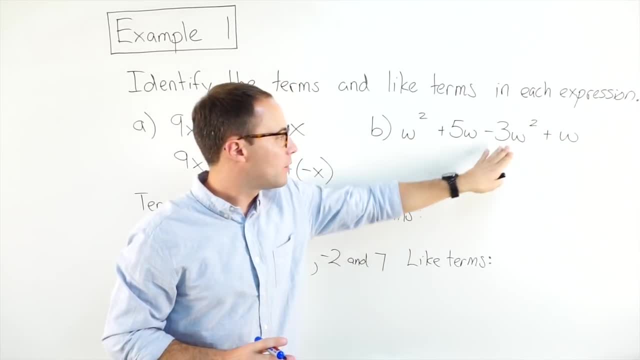 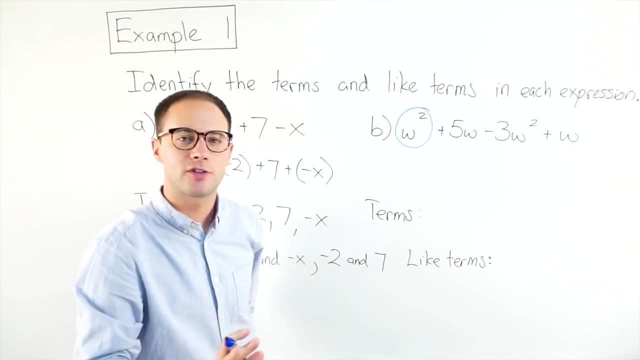 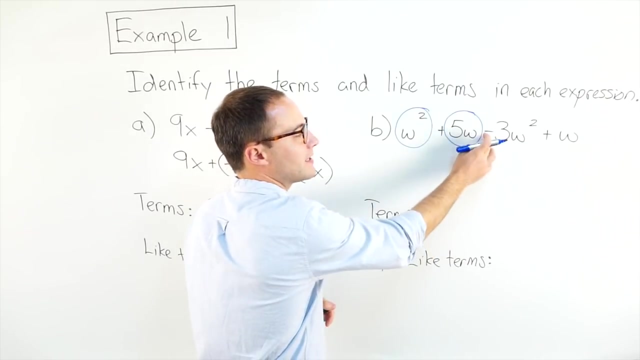 in this case, right now, you include that with whatever's after it. So I'm going to use that strategy here. So I have w squared whenever I see a plus. I'm not going to write that down, I'm not going to circle that I have a five w. I have minus three w squared. So I'm going to circle when I see 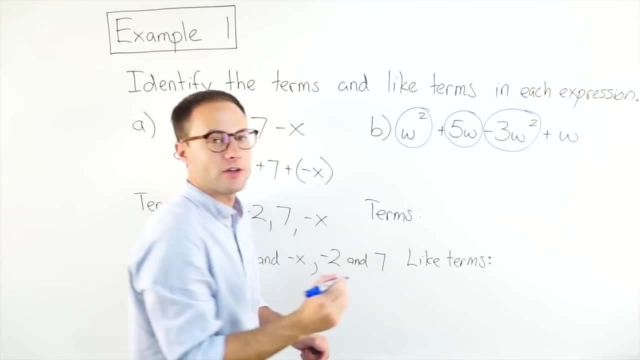 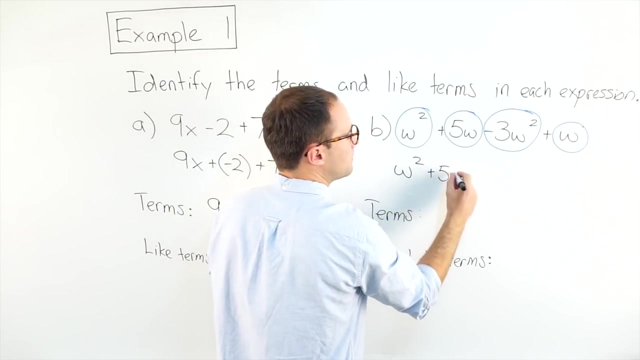 that subtraction. I'm going to include that with what comes after it, And then I'm going to have that w. Now I want you to see how it's similar to what we did here. If I change this expression to an addition expression, this is what I would get. I would get w squared plus five w, And then 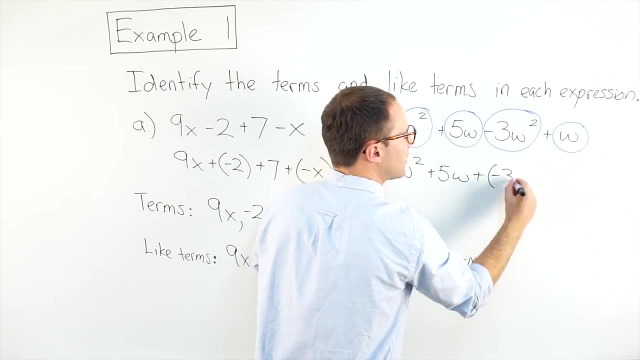 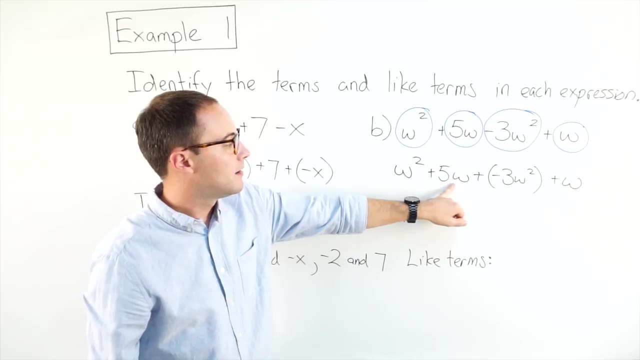 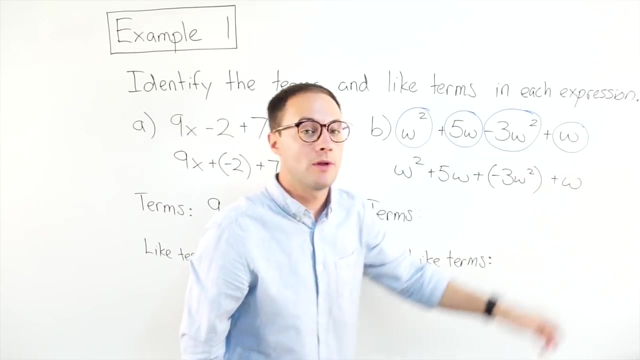 remember subtraction. we would change that to plus a negative three w squared and then plus w Again, notice my terms: w squared w squared five w, five w negative, three w squared negative three w squared w and w. So a lot of students like to use this And 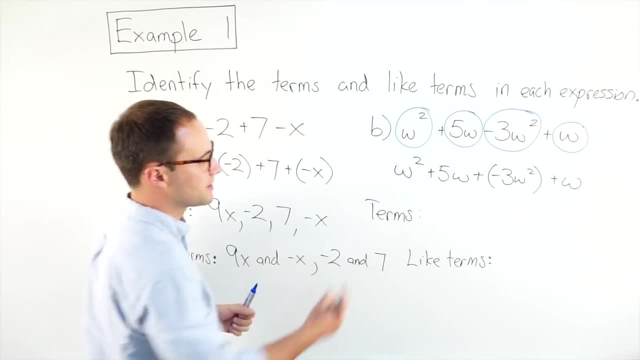 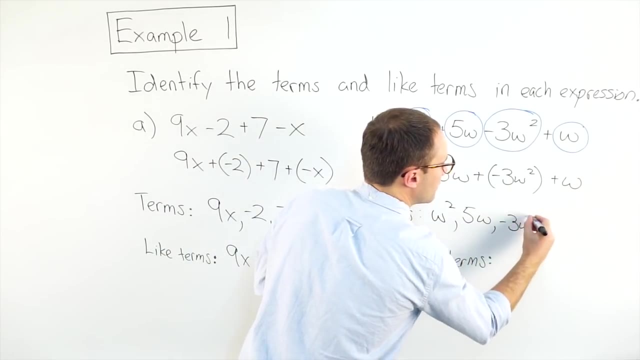 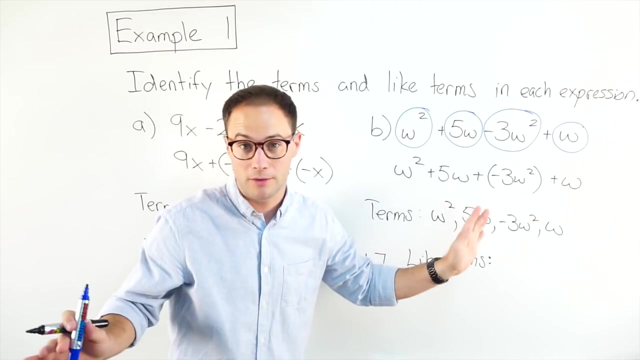 if that works for you, then great. So let's list our terms. We have w squared, five w negative, three w squared and w. Now let's do our like terms. So again we're looking. if you notice they're all w. But then 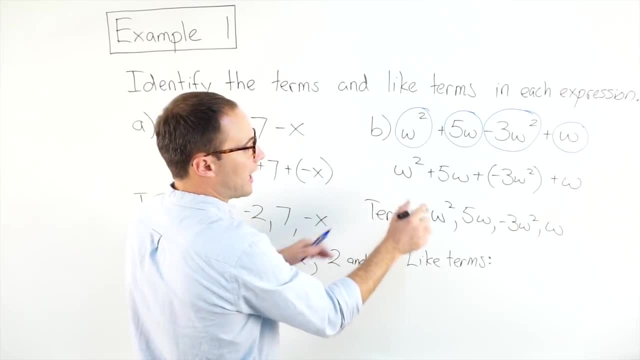 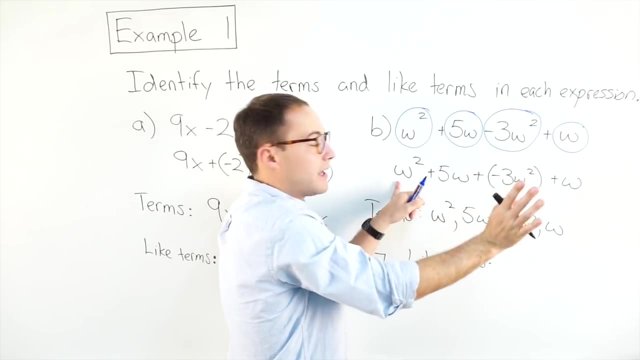 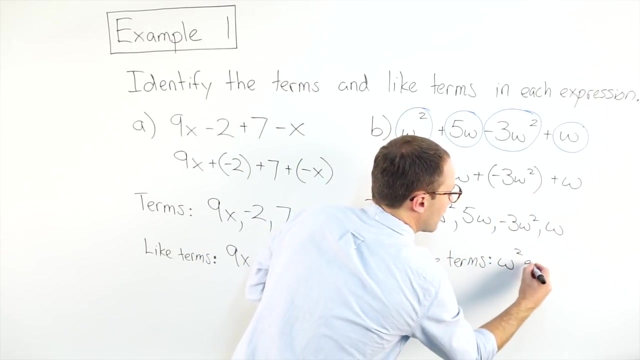 we also have to check to make sure they have the same exponents. So I've got a w squared here and a negative three w squared here. It doesn't matter with this coefficient, That's okay. These are still like terms because they're w squared. So that's my first w squared and negative three w. 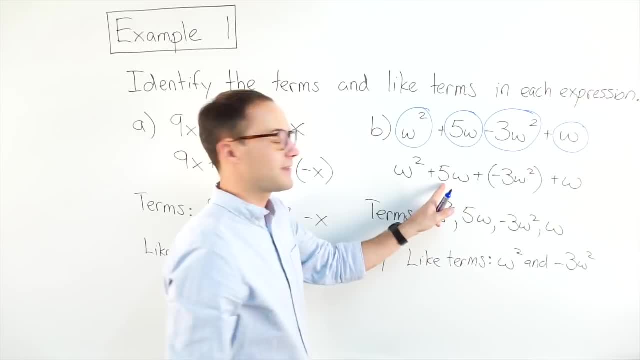 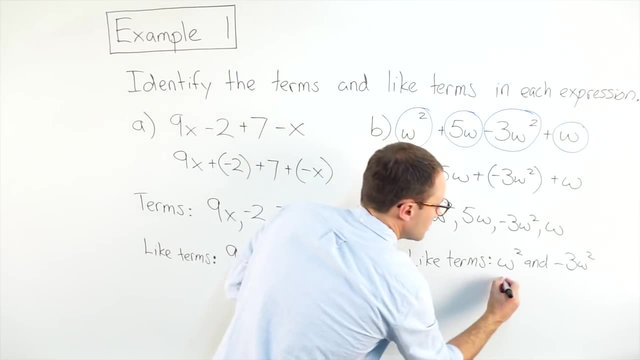 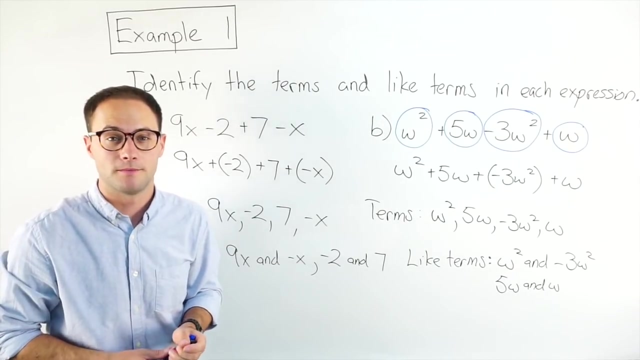 squared And then we've got five w and w. Again, the coefficient is negative. three w squared, The coefficient is okay. We're just looking at the same variable, In this case the rates of the first power. So five w and w, Those are my other like terms. Let's look at another example: All. 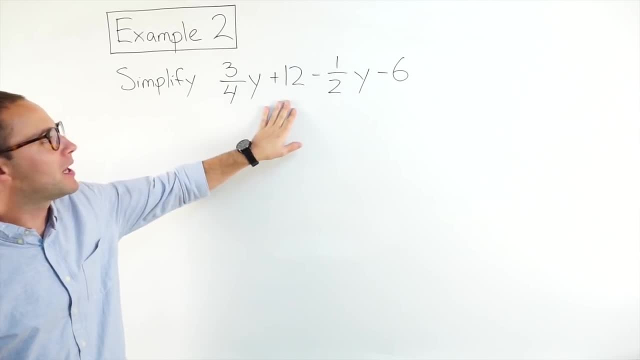 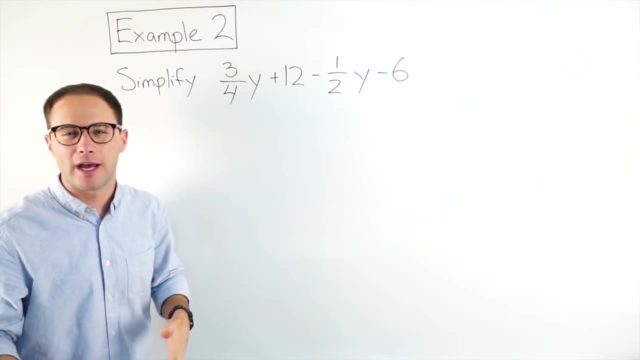 right. example: two: simplify three: fourths y plus 12 minus one, half y minus six. Okay, Well, first I know how to simplify fractions. right, Two, six would become one third. But what about simplifying algebraic expressions? How do I know? when it's in simplest form, When there are no like terms and no? 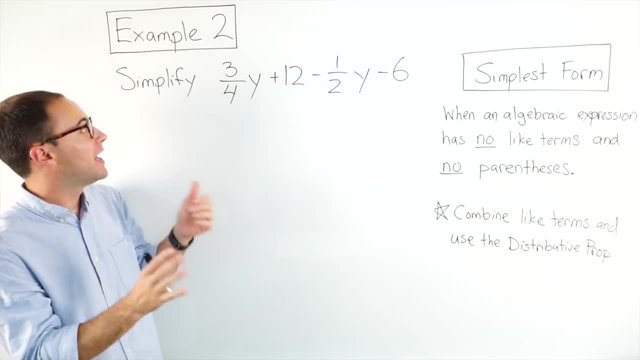 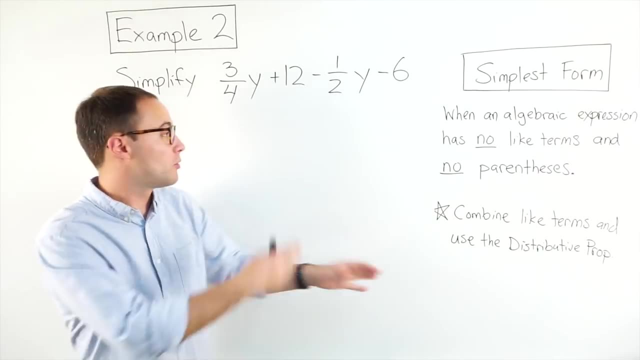 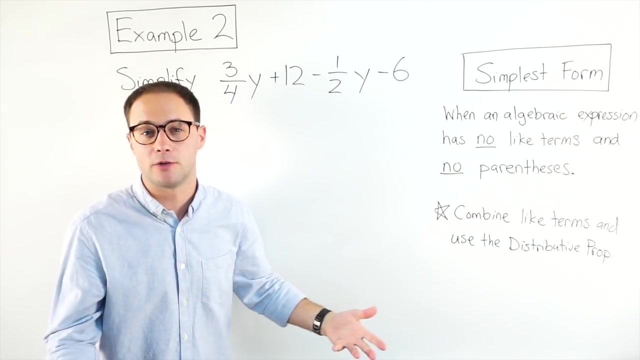 parentheses. When you get to that point, then you've simplified it far enough. it's in simplest form And to get there, we call it combining like terms. So what we just identified, when you see like terms, we can combine them And use a distributive property when you need to. That's. 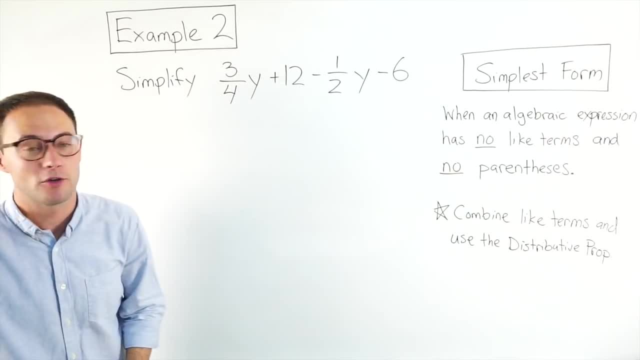 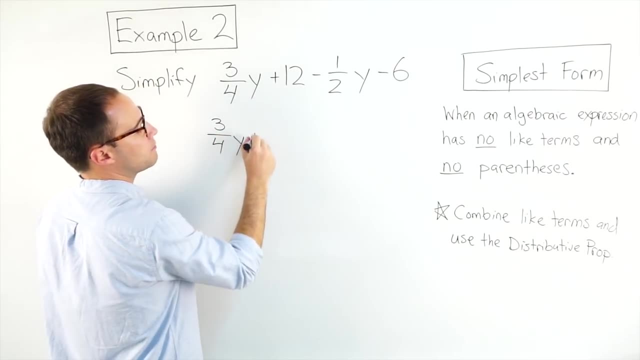 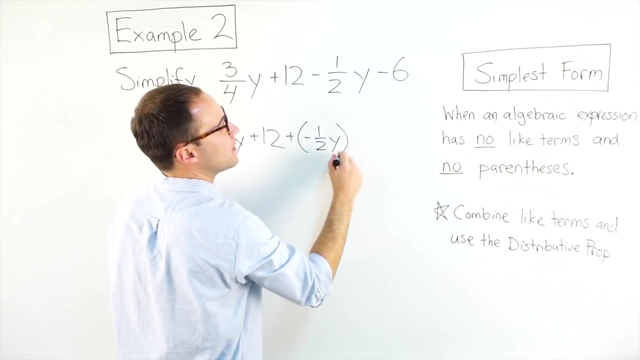 going to help you get rid of the parentheses, So let's try example two. I'm going to change it to an addition expression. So this is going to become three fourths y plus 12.. That's already addition. This minus is going to be plus a negative one half y And then that minus. 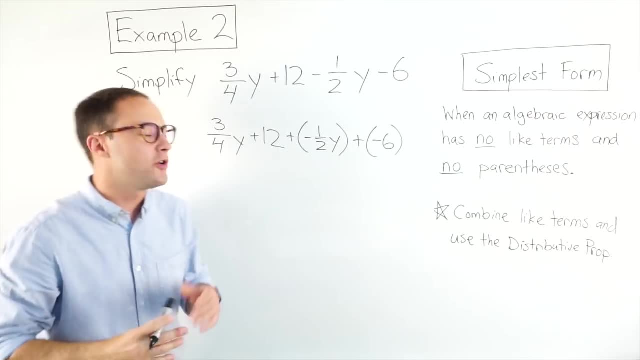 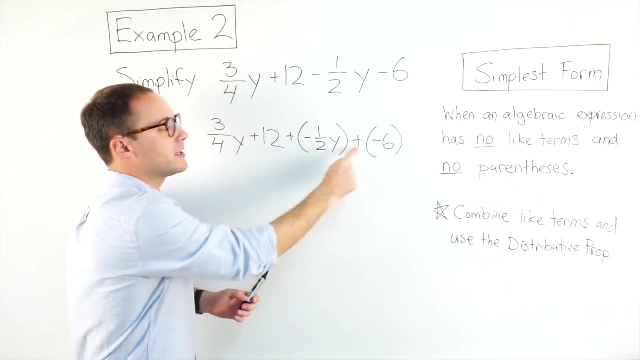 six becomes plus negative six, And the reason we do that is because now I can change the order. the commutative property of addition means I can change the order around because I have all addition. So I'm going to rewrite it: three fourths y switch this around. 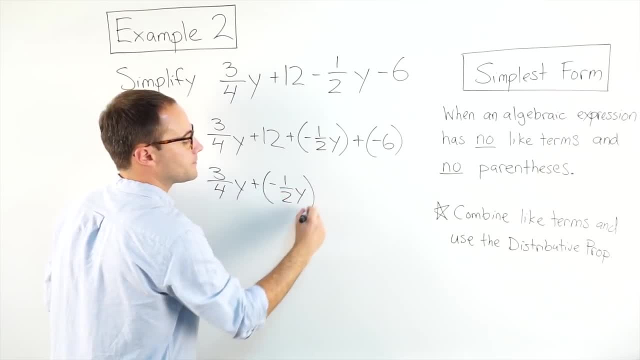 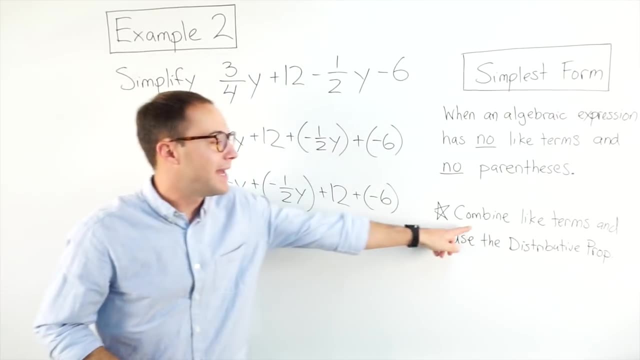 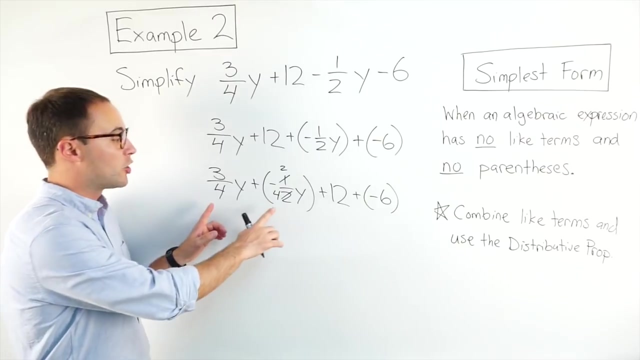 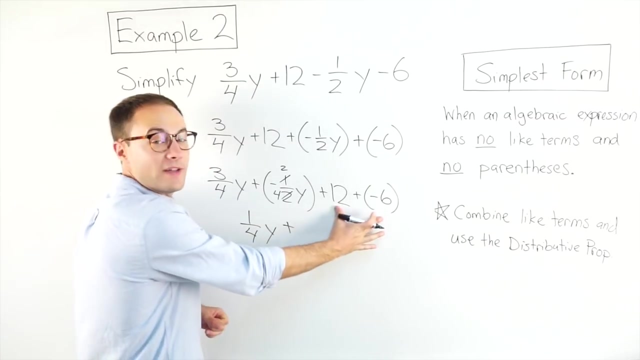 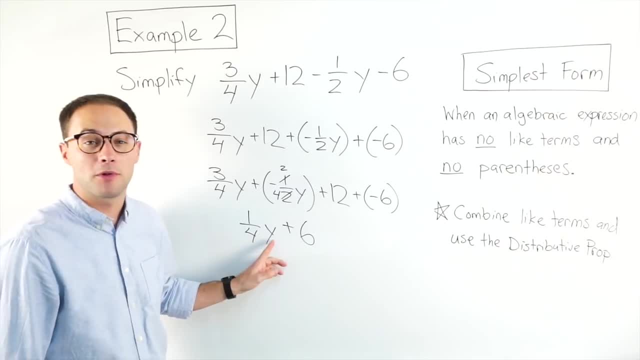 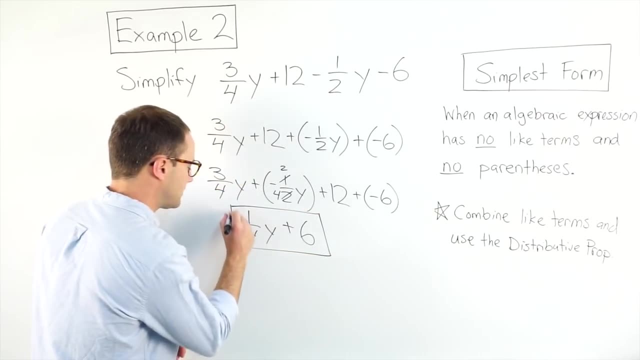 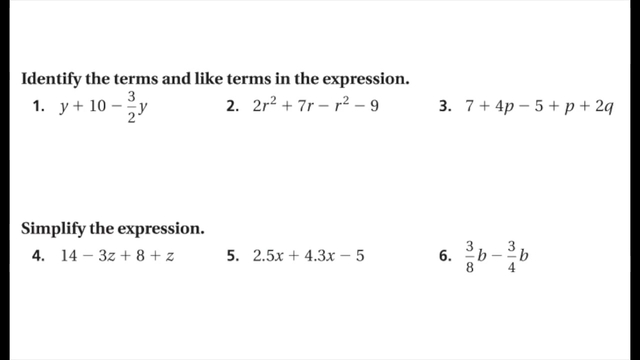 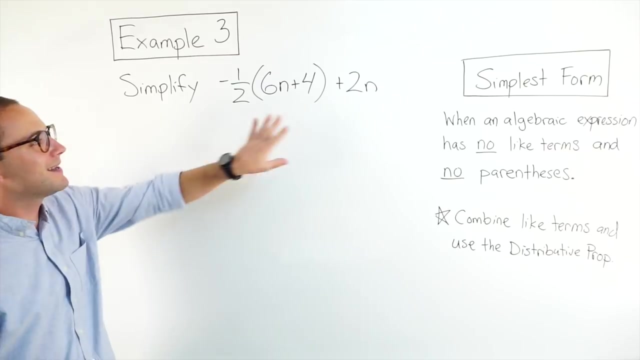 No, that's a constant And that has a variable of y. They're not like terms. Are there any parentheses? Nope, Which means this expression here is now in simplest form. Here's some to try on your own. All right, for the last example. simplify this expression Now again to get it. 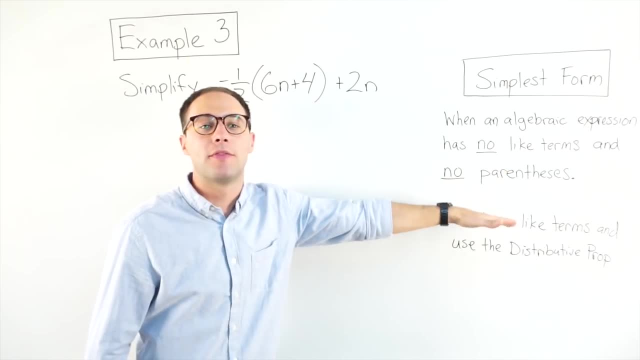 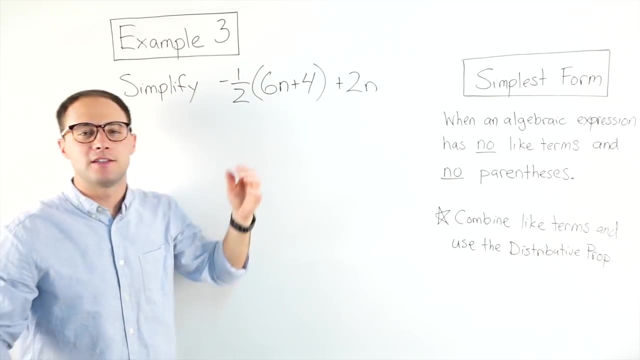 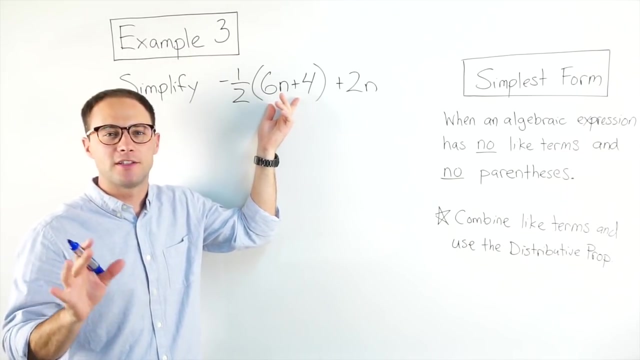 in simplest form. we're looking for no like terms and no parentheses And to get there, we combine like terms and use the distributive property when necessary. Whenever you have parentheses, first thing to always look for- and if you want to put a big star next to this, see if you can simplify in the parentheses first. 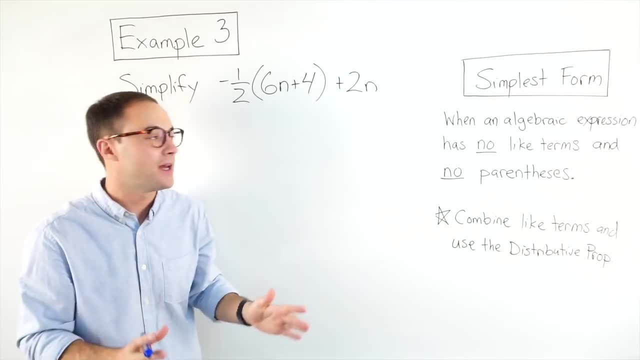 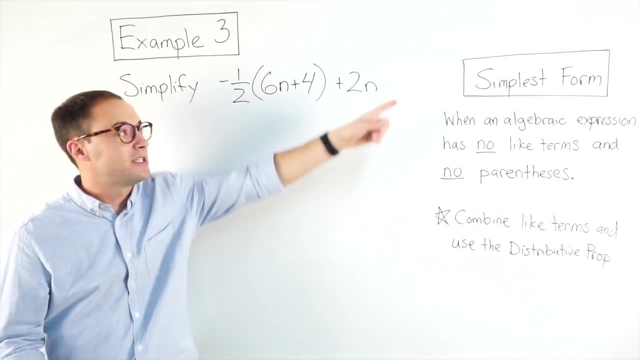 Six and plus four. I can't, they're not like terms, So that's okay. So now here, hopefully you recognize you're going to use that distributive property And if you don't remember how to do that, check out this video. but we're going to distribute. 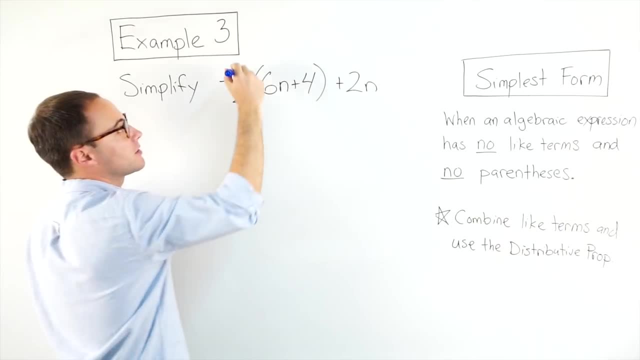 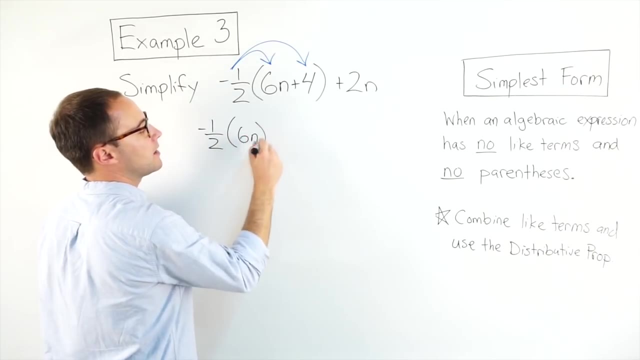 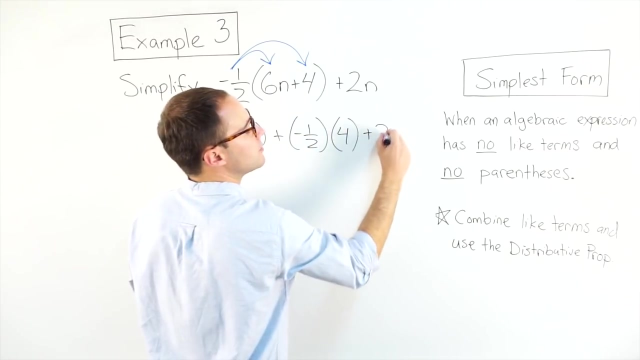 This negative one half to everything inside the parentheses first. So negative one half times six and negative one half times four. negative one half times six n plus negative one half times four, And then we still have that plus two n. Make sure you always show your work going down nice and